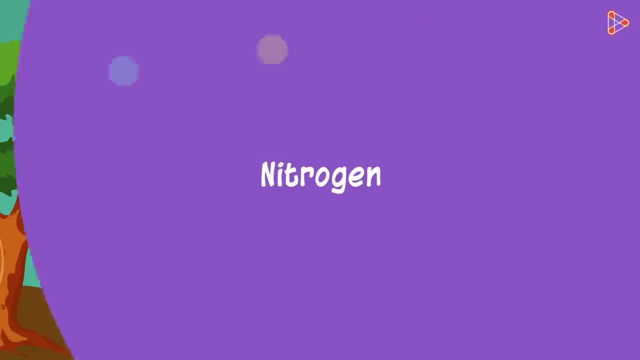 form. One such example is that of nitrogen. Yes, atmospheric nitrogen is extremely important for the proper functioning of cells. The main reason for that is that proteins are made up of amino acids, which are in turn made up of nitrogen molecules. Also many other compounds. 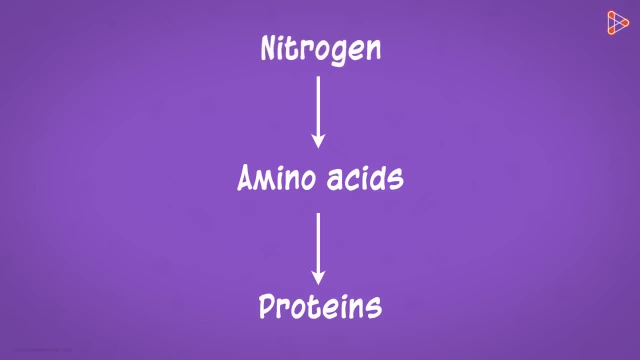 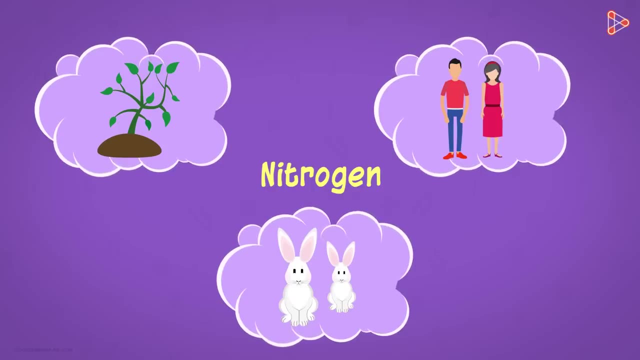 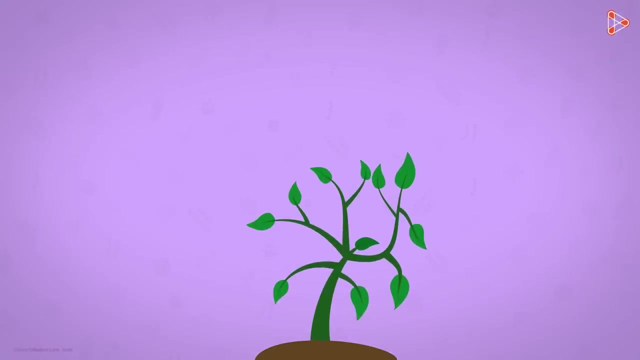 important for the cell are made up of nitrogen. So are we saying that nitrogen is required by all organisms? Of course, yes, But we can't really breathe nitrogen from the air. So this problem will be fixed by the plants for us. Yes, they will synthesise compounds having nitrogen, And when we consume plants, the 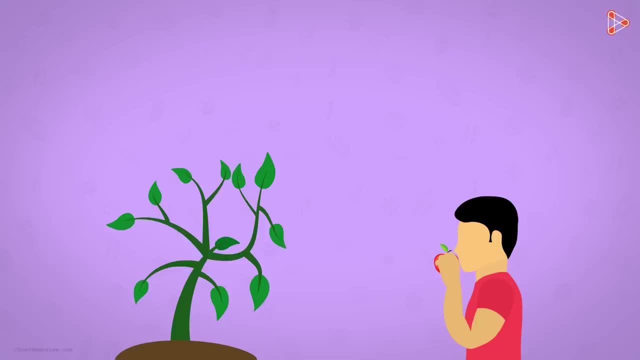 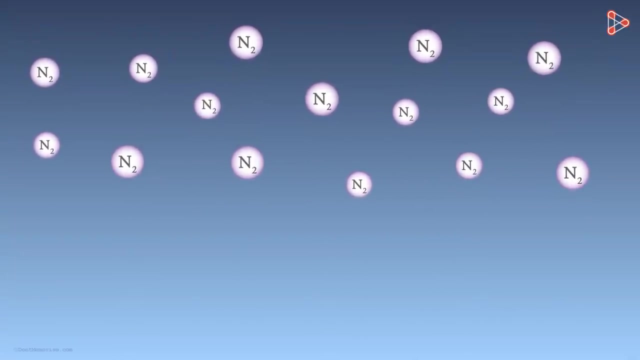 nitrogen will enter our body. Simple, isn't it? Actually, not Problem of nitrogen consumption by animals got solved, But what about the problem of nitrogen consumption by plants? Nitrogen is present in abundance in the atmosphere. However, the divalent molecule has a very strong triple bond shared between its 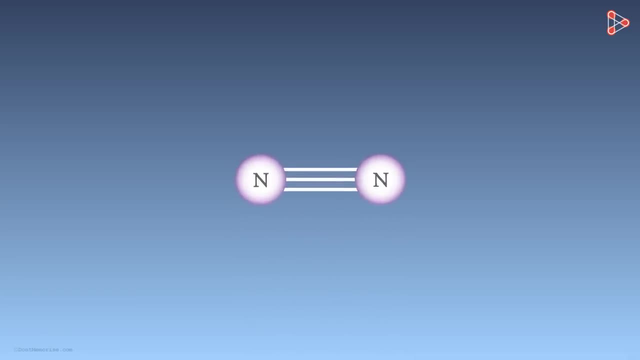 atoms, and it is very difficult to break this bond. It requires extremely high amounts of energy. One instance occurring naturally is the lightening process which helps break the two atoms apart, But that doesn't always help, So the problem still exists. Even plants cannot take in nitrogen directly from the air. 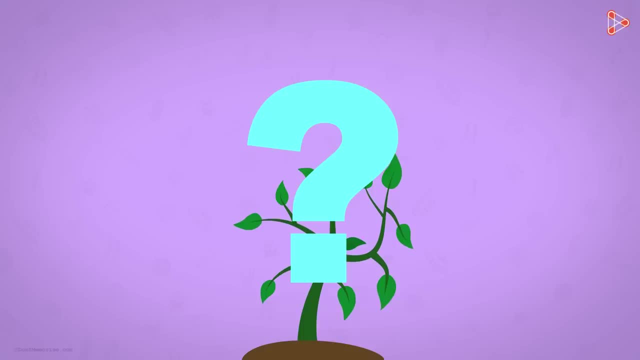 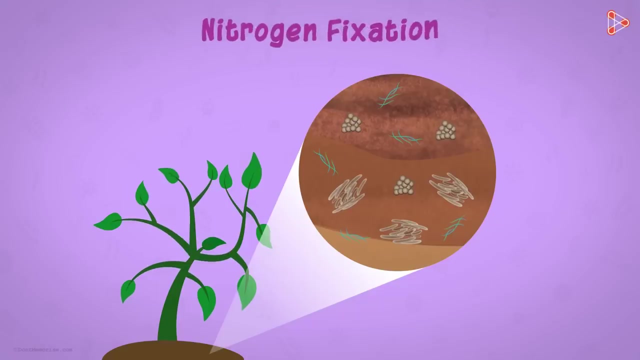 So now, who will solve this problem? We don't need to worry. Plants also seek the help of some other organisms, the microorganisms- Yes, several bacteria and blue-green algae are a part of this activity. This important process is referred to as nitrogen fixation. 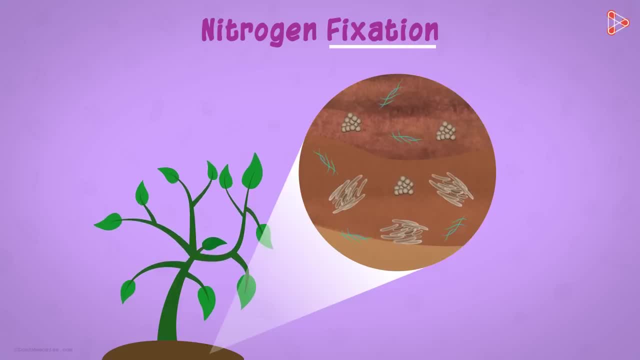 What do we exactly mean by this? The term fixation refers to converting an element into its usable form. So are we saying that these organisms convert nitrogen into utilisable forms? Absolutely, These organisms are referred to as nitrogen fixing organisms. These nitrogen fixers present in soil convert the atmospheric nitrogen molecules into compounds. 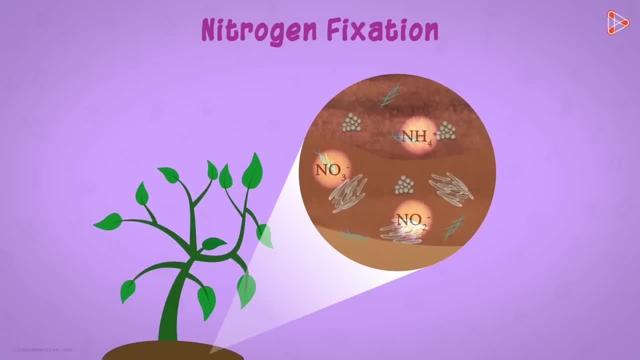 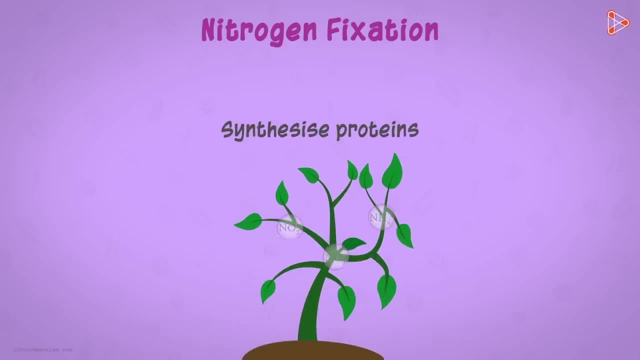 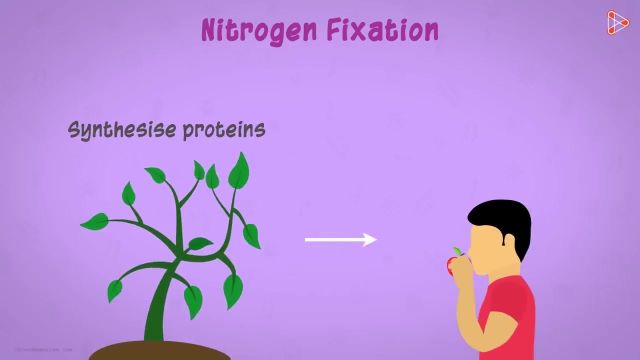 like nitrates, nitrites and ammonium. These compounds are then taken up by the roots of the plants, And then the plant uses these compounds to synthesize their own proteins. Consumption of these plants by animals and humans then gets the nitrogen into the animal. 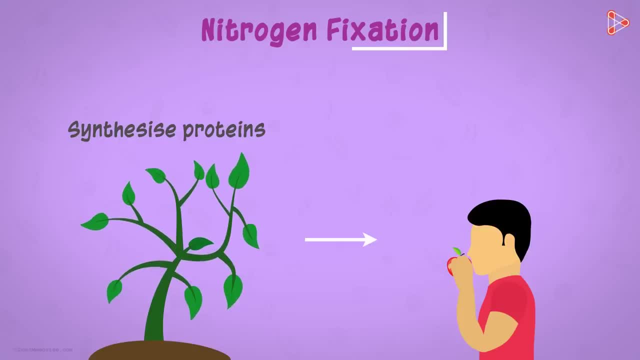 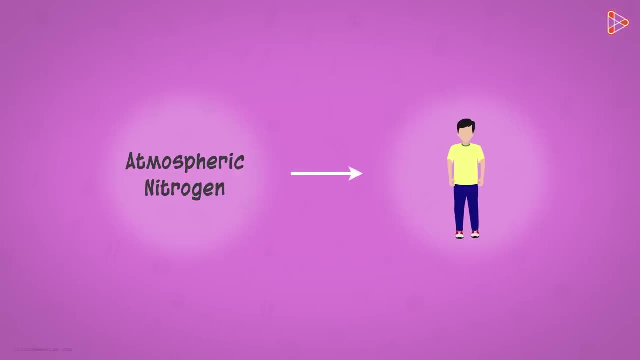 kingdom. This is how the process of nitrogen fixation occurs. Let me quickly recap what we learnt. Humans need nitrogen, but they can't take it directly from the atmosphere. Hence they get it from the plants. But even plants can't take it directly from the atmosphere. 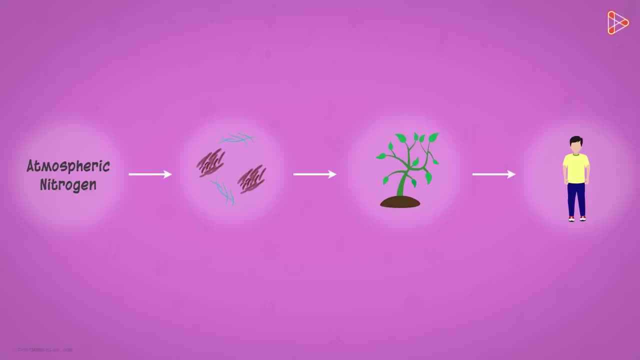 This is where the nitrogen fixing organisms come into the picture. They convert nitrogen directly from the atmosphere. They convert the atmospheric nitrogen into consumable compounds for the plants, And then animals consume the plants to get this nitrogen. But wait If all the nitrogen in the atmosphere is gradually fixed by these microbes and used by plants? 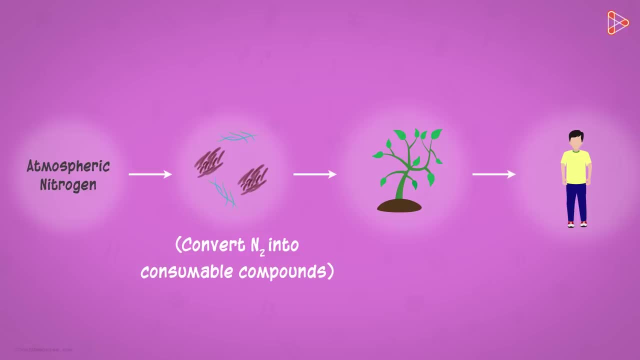 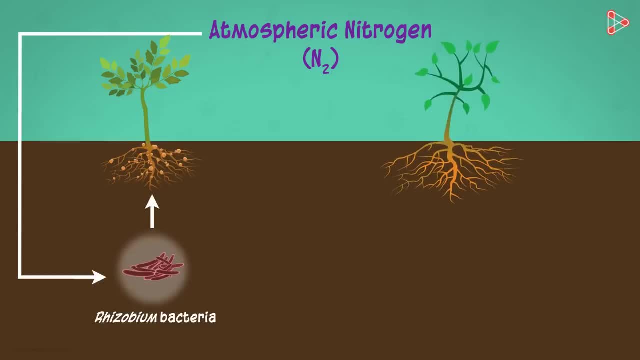 Nature, as always, holds a secret solution. Nature, as always, holds a secret solution. Nature, as always, holds a secret solution. We don't need to worry. We have the second method: The nitrogen-fixing bacteria in the soil.